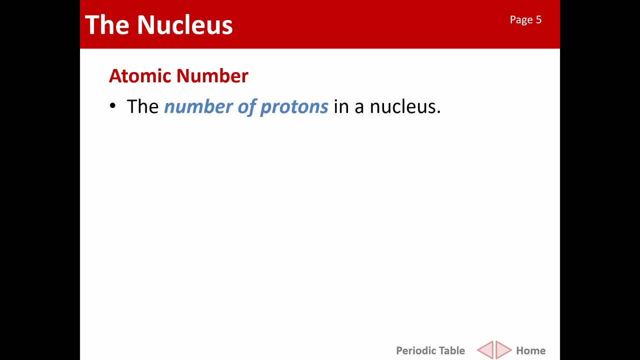 is the number of protons in a nucleus. Really it's going to define the chemistry of any particular atom. So hydrogen has one proton, helium has two, lithium has three, and so on. Every single element has a different number of protons and we call that the atomic. 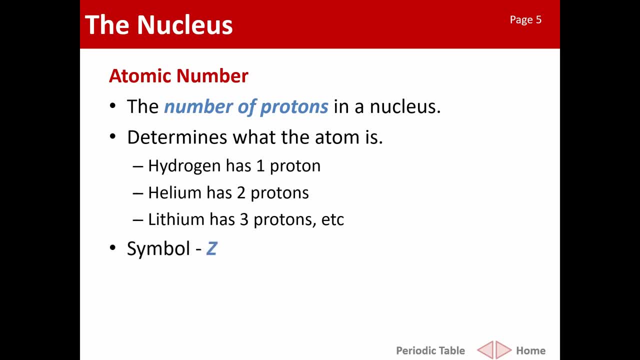 number. We give that the symbol Z, which is a bit counterintuitive. You think A, but no Z is what's used for that. The mass number is the second number that you'd see in a periodic table. It's usually a larger number and that is the number of protons plus neutrons in a nucleus. So it always. 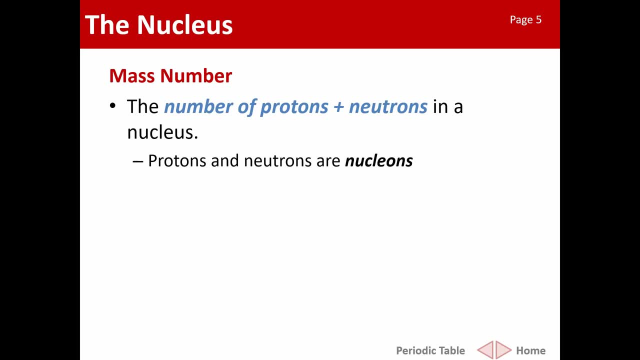 has to be at least the size of the atomic number, And usually bigger because there are extra neutrons as well. Together, protons and neutrons are called nucleons, So sometimes you might see that written down as a nucleon number And again, counterintuitively, it has a symbol that doesn't seem to match up with its name. We. 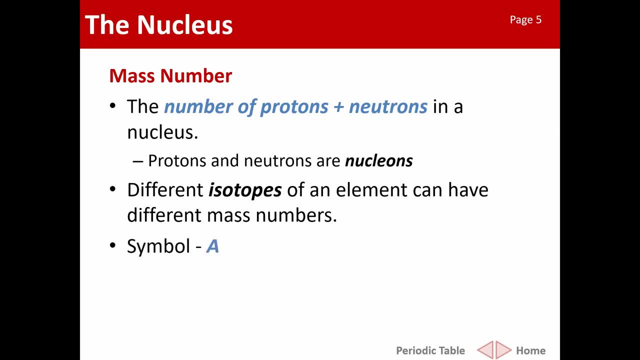 give it A This word isotopes appears. An isotope or different isotopes of an atom are different versions of the atom that have the same number of protons and therefore they're the same chemical element. different numbers of neutrons, and we'll come back to that in a second. 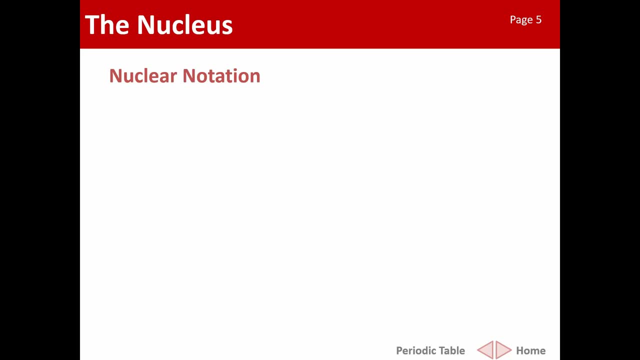 Whenever we write down a symbol to represent a nucleus, we use this formation, where a is the mass number, z is the atomic number and x is the chemical symbol. We always put the mass number- the larger number- on the top and the smaller number- the atomic number- on the bottom. 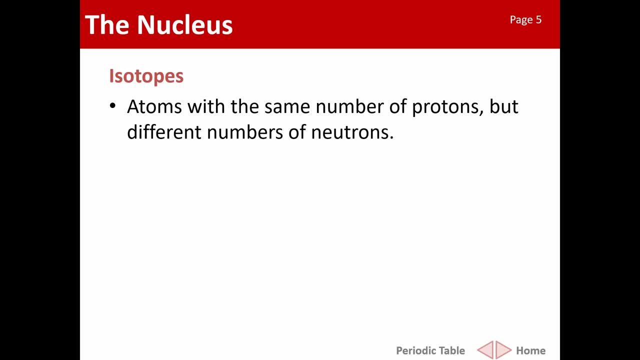 So we'll see some examples of that when we look at isotopes. So isotopes, as we said, are the same number of protons, different numbers of neutrons. That means that they have the same atomic number, the same mass number. 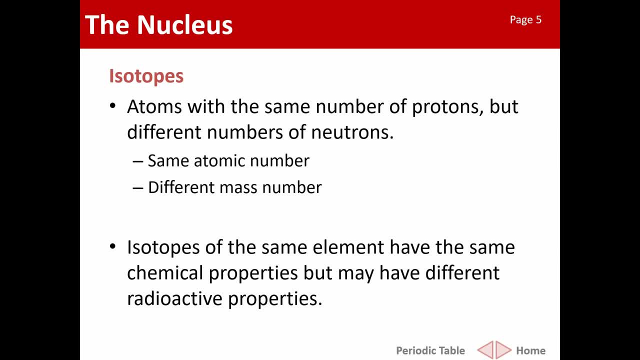 and because they've got the same atomic number, the same number of protons, they also have the same number of electrons, which means that their chemical properties are identical. So, for example, you could have different versions of carbon, and you know they can. they can swap with each other in a chemical reaction. 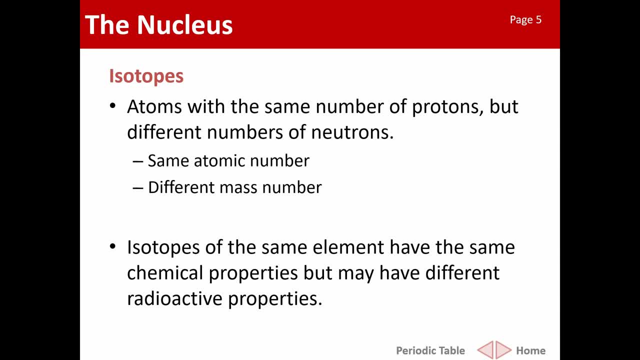 without causing any difficulty. So some of the carbon in your body is what we call carbon 12, a certain percentage will be carbon 14.. Chemically they do exactly the same thing. They will have differences when it comes to the radioactive properties which we'll 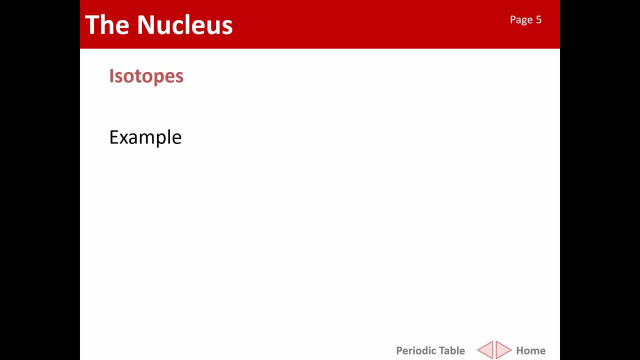 come to at a later stage. An example: helium-4 is our normal helium. It has two protons and two neutrons, so it's got an atomic number of two on the bottom, a mass number of four on the top. Notice I called it helium-4.. 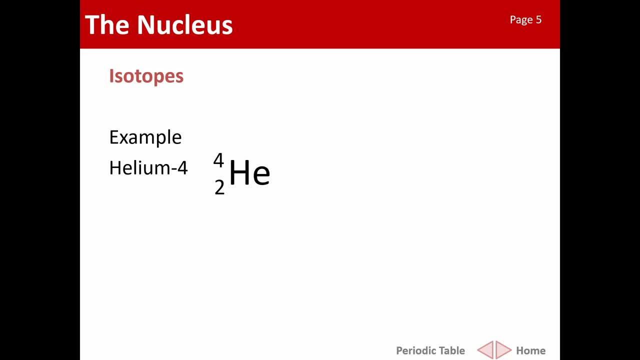 If you ever hear a number after an element's name, that's referring to the specific isotope. So helium-4 is a mass number of four. But we can also have the rarer version, helium-3,, which has two protons, one neutron and two neutrons. 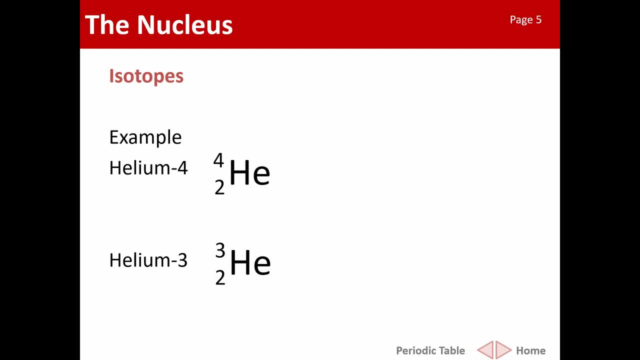 But we can also have the rarer version, helium-3,, which has two protons, one neutron and two neutrons For an overall mass number of three. Some isotopes are not stable. A lot of isotopes are stable, but a fair 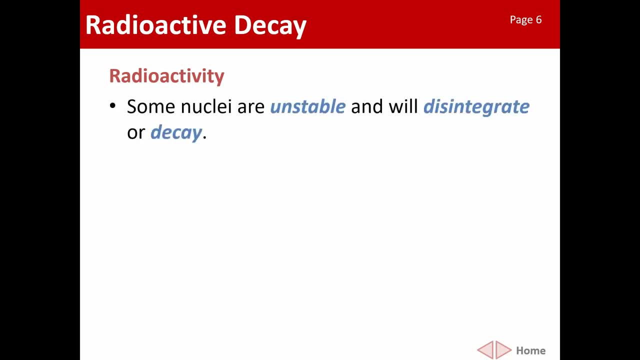 number are not stable and will tend to disintegrate or decay. In other words, they've got too much energy and the combination of protons and neutrons in the nucleus are not quite balanced. And to make itself more stable. and to make itself more stable. 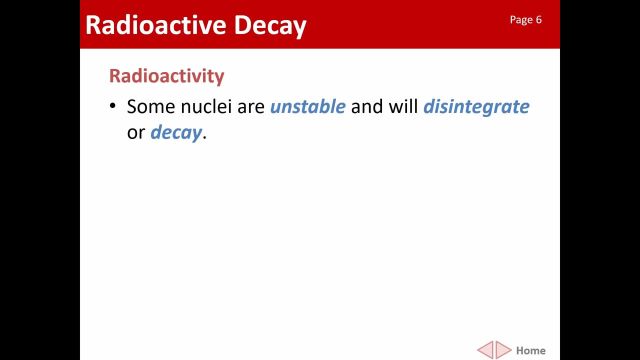 the nucleus will tend to sort of split apart and give off extra bits, And these extra bits that come off are known as ionizing radiation, And we'll see why they're called ionizing a little bit later. Any nucleus that does tend to want to decay. 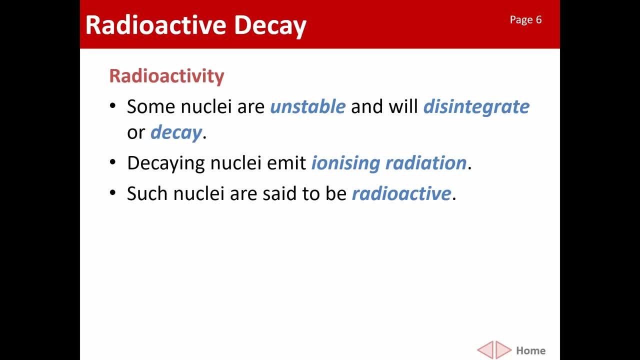 we'll call that a radioactive nucleus Activity refers to how much radiation is coming out or how many decays there are. Now we mentioned this in class When we did the DICE experiment. Radioactive decay is both random and spontaneous. These are important key words, you know. 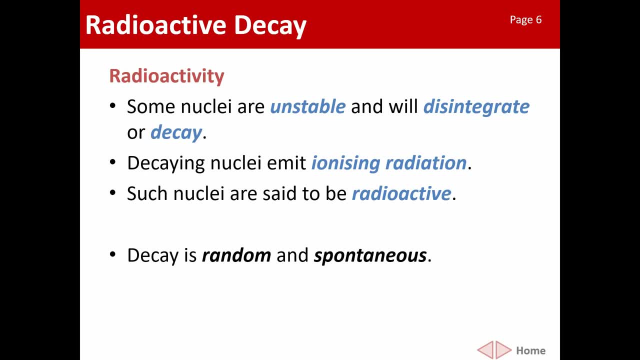 Random implies that you cannot tell when any particular nucleus is going to decay, Nor can you make it decay. You can't heat it up or add electric charge or add some sort of chemical to make it decay. It'll happen by itself in its own time. 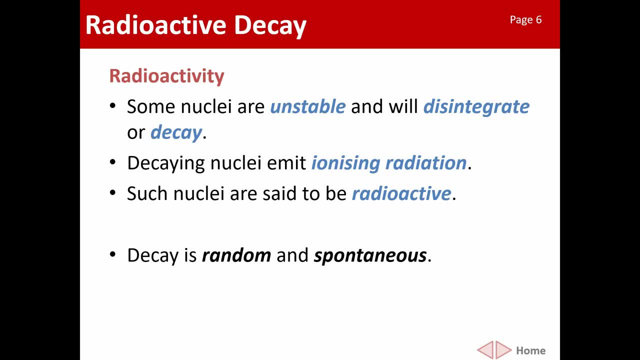 And you cannot predict when it's going to happen. You could have two nuclei identical beside one another, another and one might decay in the next 10 seconds and one might not decay for another 10 years. There's no way of knowing Spontaneous means. it'll happen by 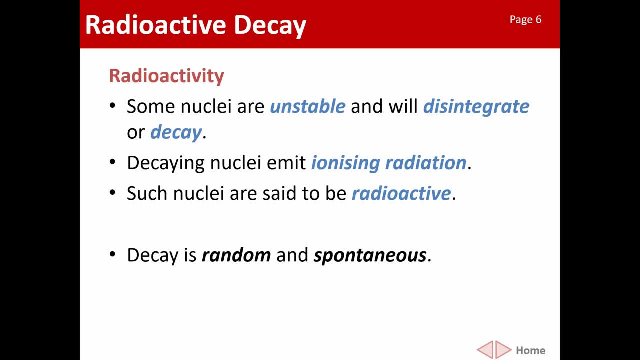 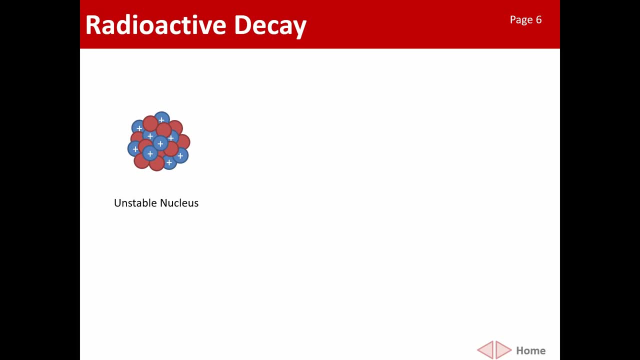 itself. You cannot make it happen So random will happen, unpredictably Spontaneous. you cannot make it happen So generally what happens is you've got an unstable nucleus, It's got too many protons or too many neutrons, and what tends to happen is it'll try to get rid of some of its excess energy, usually by 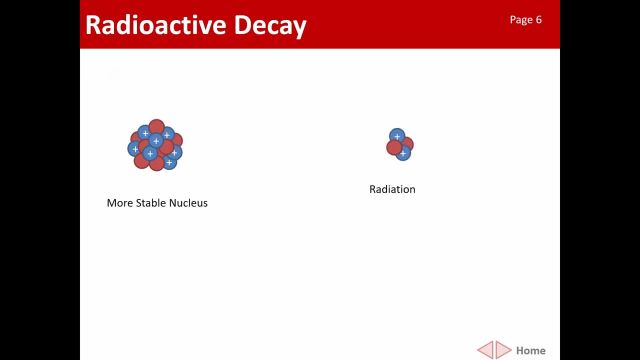 splitting off a particle. In this case we've got two protons and two neutrons coming off, leaving a slightly smaller, more stable nucleus behind and this ejected bit of particle, which is radiation. The word radiation just means to radiate out some sort of energy or particles that are going to come out. 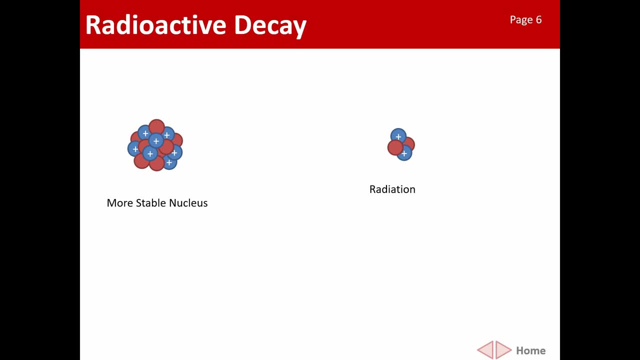 from something. In this case, we are interested in types of radiation known as ionising radiation. That type of particle with two protons and two neutrons is known as an alpha particle, and we'll have a look at what that means at a later stage. It's important to remember that we don't talk about an 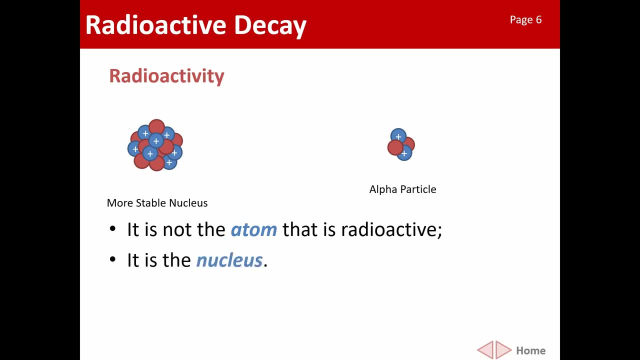 atom being radioactive, it's the nucleus that decays. This whole thing is called nuclear decay and we're always talking about the nucleus. if an atom is really sorry, if a nucleus is radioactive, it means it is going to decay and give out radiation. we can measure radioactivity using something called a geiger-muller tube and i'll show you. 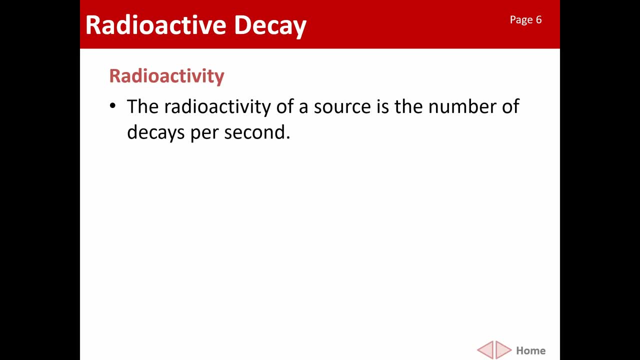 one of those in a bit and it will decay, detect how many decays or how many bits of ionizing radiation come into it, and if we count the number of decays per second, that is what is known as the radioactivity of a source. the unit is the becquerel. so if something had a radioactivity of three, 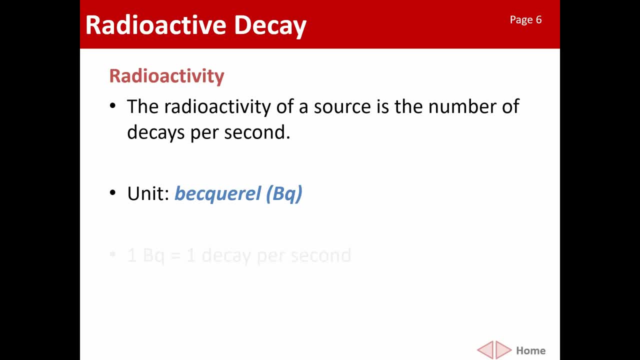 becquerel, it would mean three decays per second. a thousand becquerel, a thousand decays per second. we have three main types of alpha of. we have three main types of ionizing radiation that we're concerned with in this topic. the first one is known as alpha radiation. 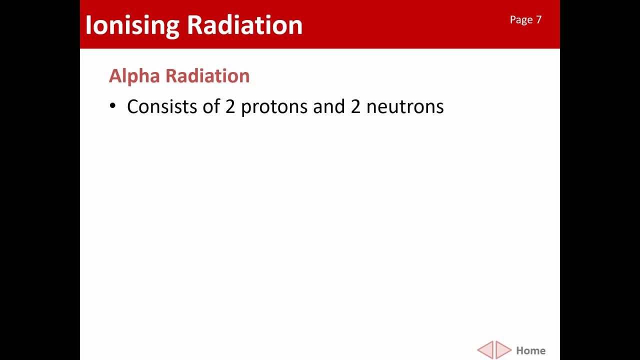 alpha radiation, as i've mentioned already, consists of two protons and two neutrons. that means we can give an atomic number of two a mass number of four. so really it's the same as a helium nucleus, but it doesn't have any electrons, it's just a particle that is split off from an unstable. 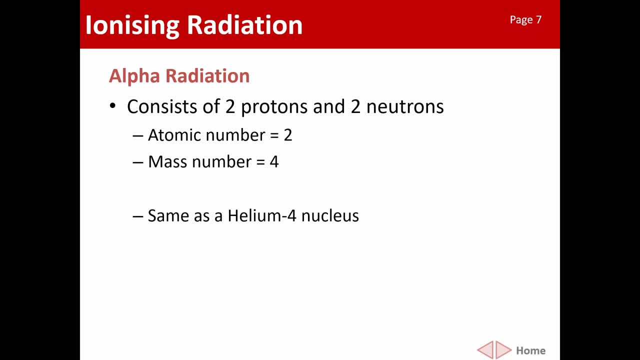 um and and leaves it, taking some energy behind it. this is the way we read it. we've got four, two and alpha. alpha is just the first letter of the greek alphabet. uh, the four refers to the mass number, the two refers to the atomic number. that formation of four, two and alpha is important. that 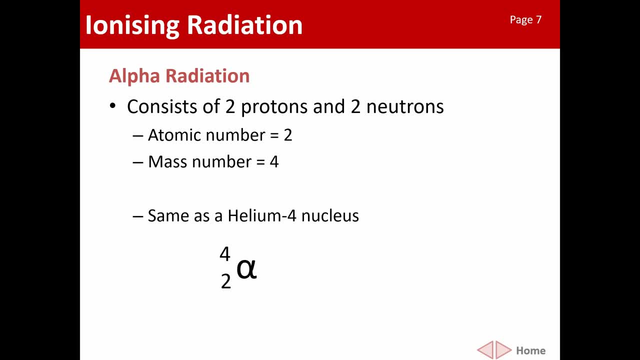 you memorize that. you will not have to memorize the notation for any other um isotopes or elements, but you do need to memorize them. for the three types of ionizing radiation. you could also write it down as 428g, because they're identical. 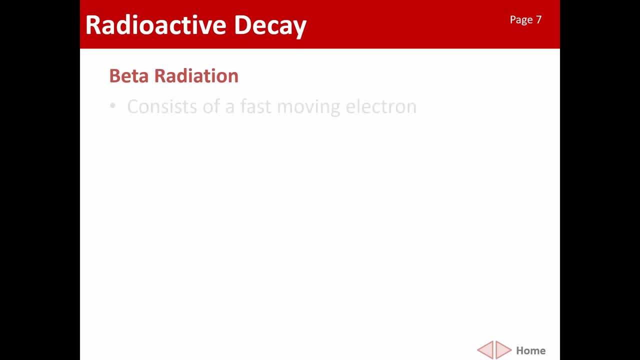 our second type is beta, or beta radiation, and it consists of a fast moving electron. now, this is not an electron that has split off from the um, the shells of an atom, or orbiting a nucleus. this is one that has been ejected from the nucleus itself, which should sound surprising, because you don't normally get electrons in a 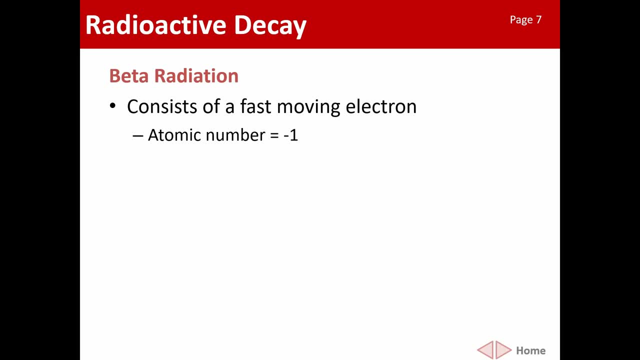 nucleus, we give it an atomic number of negative one um. it's not that it has negative one protons, but it's got the charge of negative one um. and so for the sake of uh, nuclear decay equations that will come to you in a future lesson, we're going to call that negative one. i'll refer back to that in. 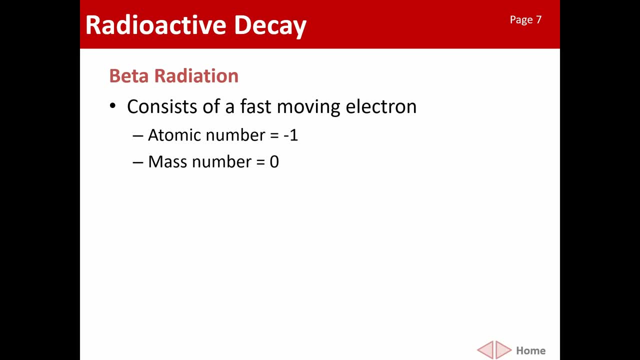 the minute right now. so we can write it down as zero, negative one and, as i said, the negative one is a mass number of zero. it doesn't mean it has a mass of zero because it's an electron, is a mass of 1 over 1840 in terms of the proton, but we could give it a mass number of zero because there are no protons. 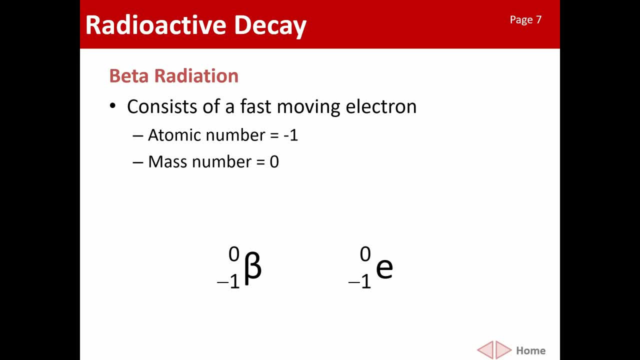 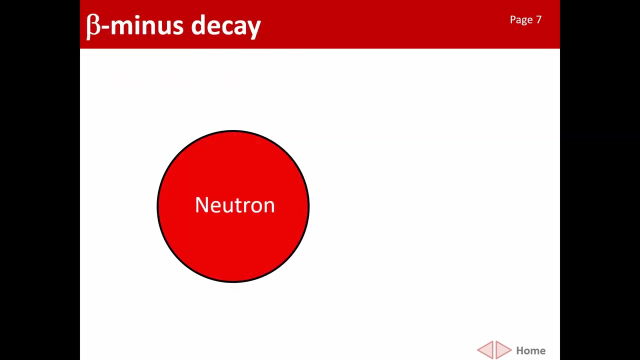 and no neutrons, and so we can write it down as zero negative one beta or zero negative one, e said, doesn't mean that it's got a negative proton. It is there because it is produced by a neutron turning into a proton. So, under certain circumstances, which we call beta minus decay- 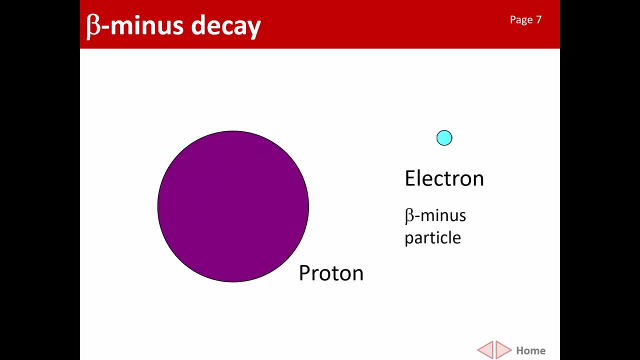 a neutron will change into a proton plus an electron. That electron is ejected. So that's this extra electron that's been generated inside a nucleus and has come out. Before that reaction there were no protons, Afterwards there is a proton, And so really to balance both sides of 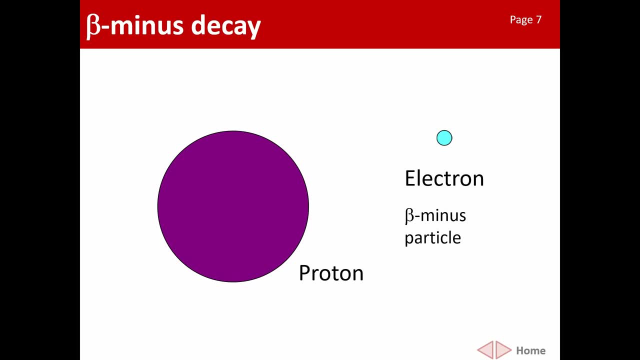 the equation, we give the electron an atomic number of minus one to balance those out. We'll see what that means. as I said at a later stage, There is another rarer form of beta decay, called beta plus decay, which you do not need to know about in this course. 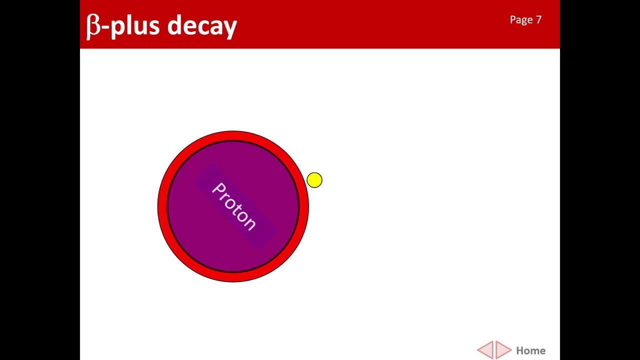 What happens is a proton will decay into a neutron and give out a positive electron, known as a positron. This is antimatter. We deal with this at a level, but it's not something that you normally see. But I'm putting it there because it shows that a neutron is not 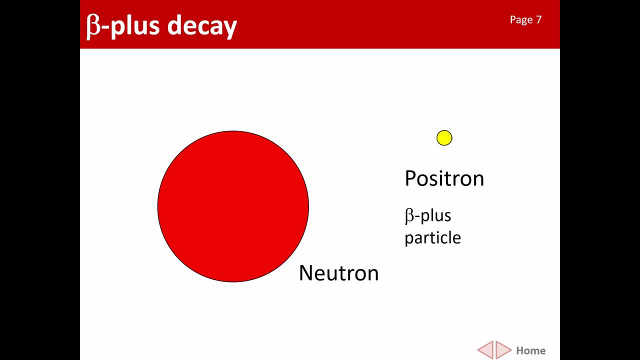 normally made up of a proton plus an electron. It just so happens that whenever it's unstable, whenever a nucleus is unstable, one way of it getting rid of extra energy is these, these particles changing from one type into another. Our third form of ionizing radiation is called gamma, And it's very different because it is 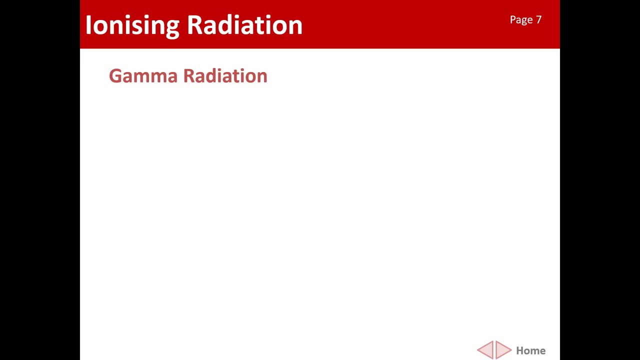 not a particle. Alpha was two protons and two neutrons, Beta was an electron. Gamma is an electromagnetic wave. It's just a burst of energy in a waveform. We'll deal with that in the first topic of unit two waves. But it's similar to light or x-rays or radio waves. 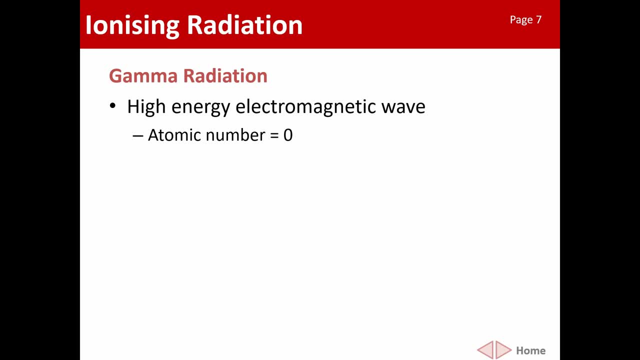 It's just a burst of energy that comes out. As such. it has no atomic number and no mass number because it is not a particle. So it actually has zero mass. The beta particle had a mass number of zero, but it did have a mass. This has no actual mass And we write it down like this: Zero. 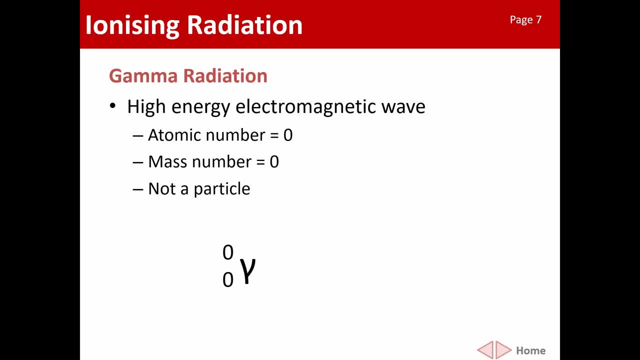 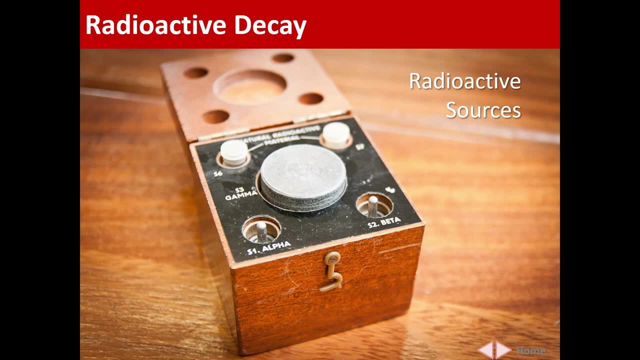 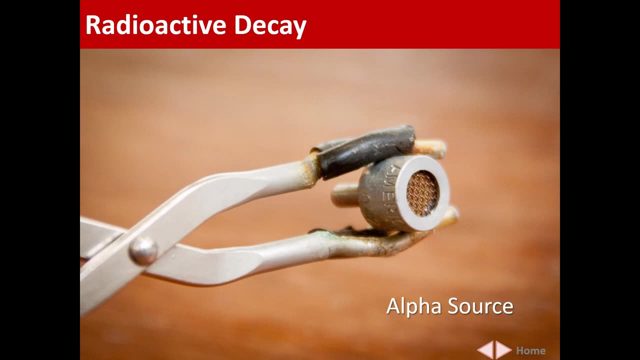 zero with this odd sort of gamma form. Whenever we're in school, we normally do experiments with this, using radioactive sources that come in little pots like this. This is called a sealed cup source And you see it's a little source of, in this case, americium-241,, which is an alpha emitter. 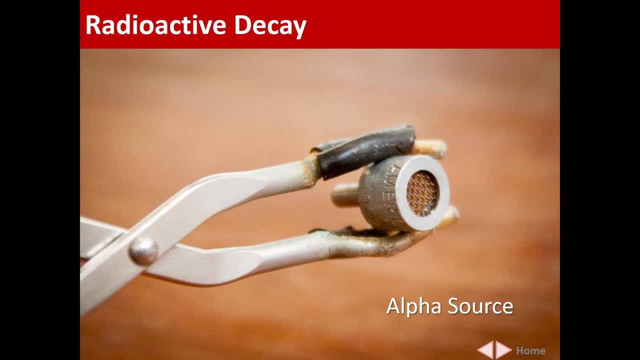 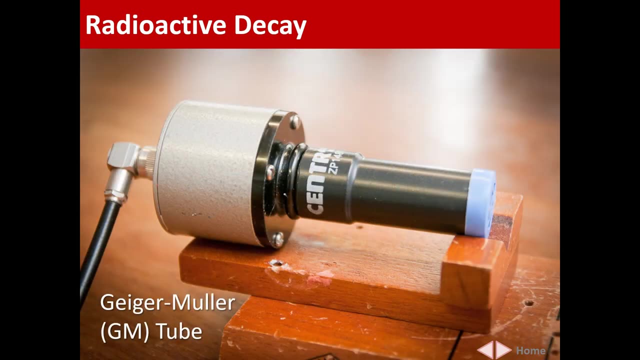 stored in a little pot with a little bit of foil behind it. I don't have any of these here at home, so you can't see experiments of these, but that's the sort of thing that we'll be using. This is a Geiger-Miller tube that we use to detect ionising radiation that we have in school. I'll 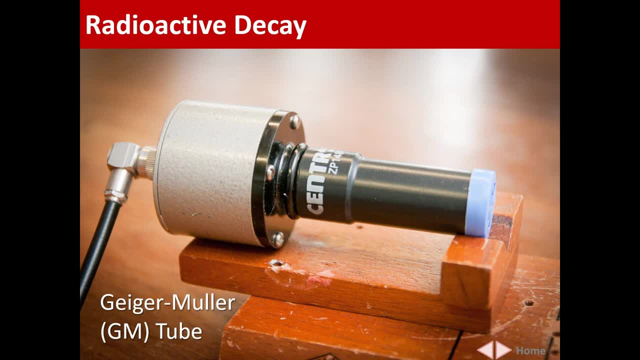 show you a different kind of one. What happens is the ionising radiation moves into it, a little current is produced and that's attached to a counter and it counts up the number of ionisations that take place And we can use that to measure the activity of a source by measuring. 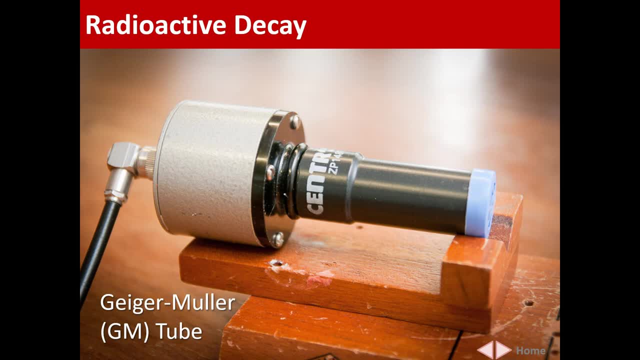 how much of the activity is produced. We've got this little laser tube that's attached to it. I'm many counts there are in a certain amount of time dividing that down to find how many counts there are per second. But sometimes we use per minute. 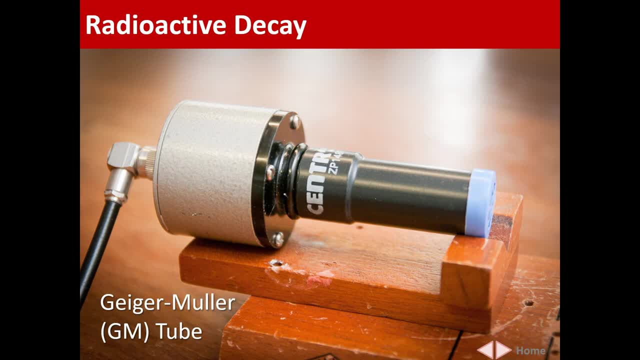 or per hour. We call it ionising radiation because the particle that comes in the alpha or beta or gamma will cause an atom, if it hits the atom, to lose an electron. So here we're going to look at an atom that has 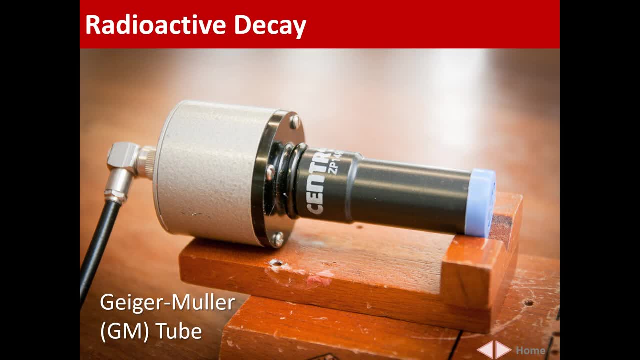 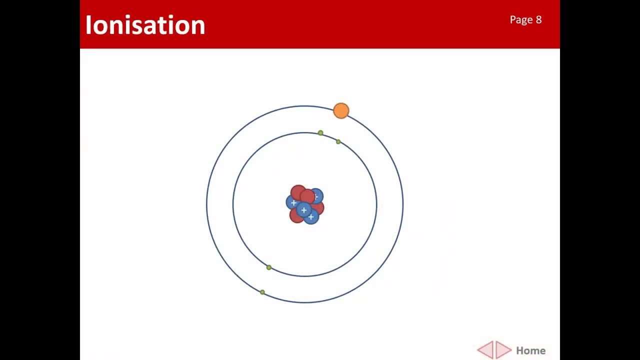 four protons, in this case four neutrons as well, and it's neutral. so it has four electrons. You can see they're all orbiting, But a particle is going to come in and it collides with the other electron and knocks it off And we're now left behind. 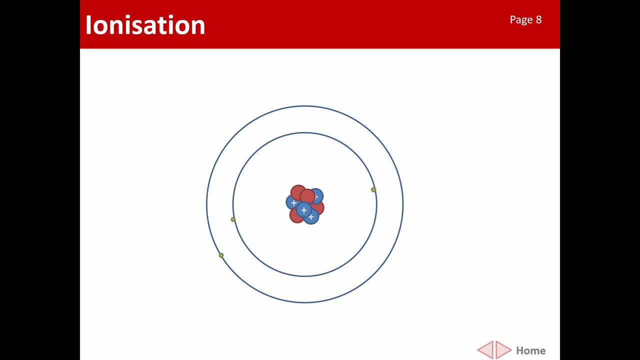 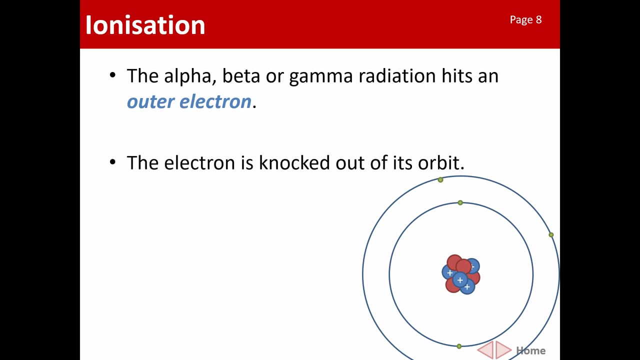 with four protons and three electrons. So in this case we're left with a charged electron. It's got one more positive charge than negative and that's called an ion. So the outer electron is hit by the alpha or beta or gamma radiation That 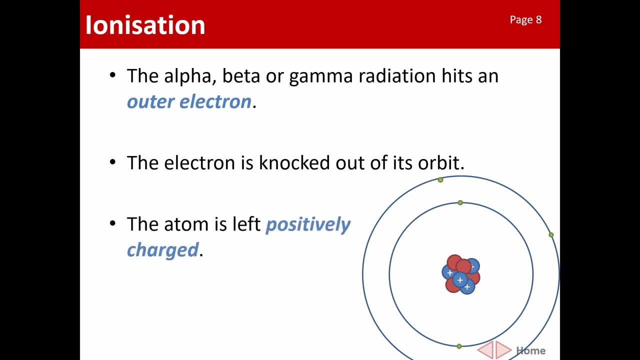 electron is knocked out of its orbit and the atom is left positively charged, And that's what we call an ion. That process is called ionisation In chemistry. you talk about ions, and they can be things that have gained or lost electrons. In this topic, we're only concerned with atoms that have lost. 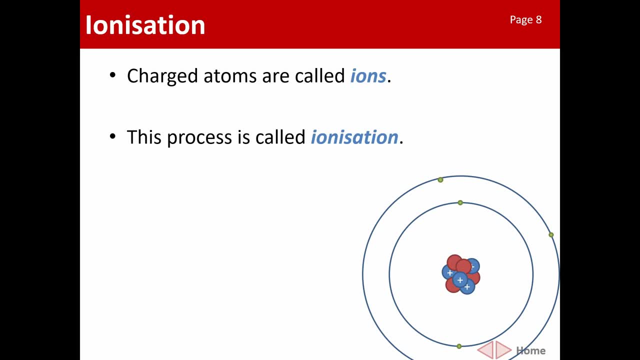 electrons. It could be an alpha particle which comes in and is positively charged and will strip the electron out of the atom. It'll try to capture electron, Or a beta particle, which is an electron, but it'll just collide and knock an electron out of the way. Or gamma radiation, as the electrons will sort of absorb the electron. 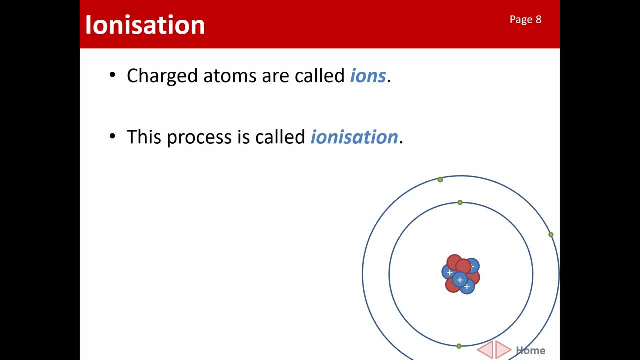 They'll absorb the gamma radiation and just be given so much energy that they break away from the atom. That's why it's known as ionising radiation. Alpha is the most ionising because it's got the biggest charge. It's also because it's the heaviest particle- it moves more slowly. 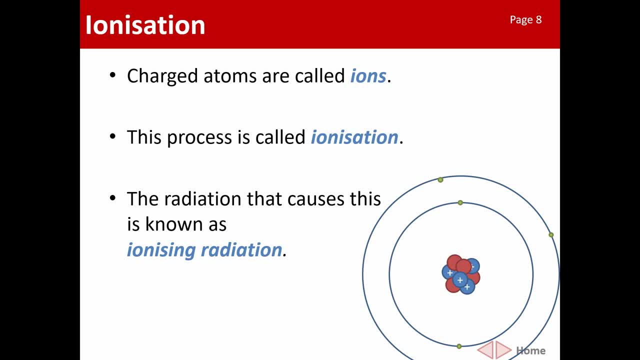 and therefore, as it moves past an atom, it has more time to collide. So alpha is the most ionising, Beta is the next most ionising. It's got less charge, Less mass. It moves much, much faster So it has less time to do it. And gamma is 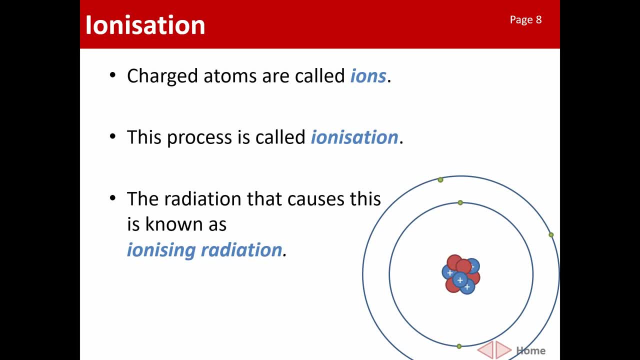 actually the least ionising because it has no mass. It has no charge, So it is less likely to knock an electron out of the atom. It can do it though, however, if the atom will absorb the gamma particle's energy, the gamma wave's energy and the